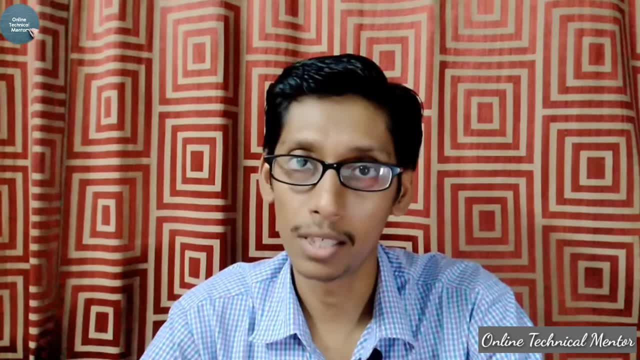 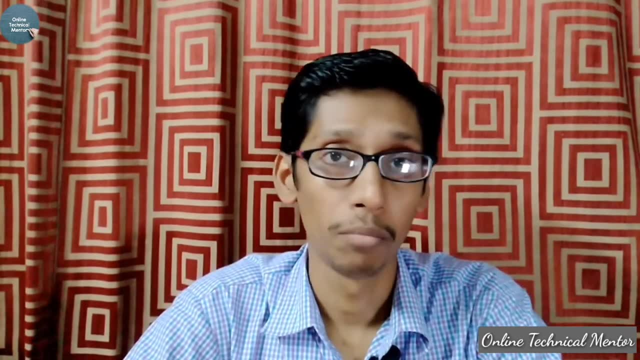 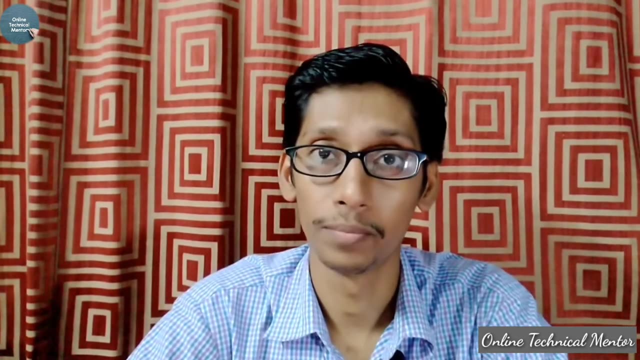 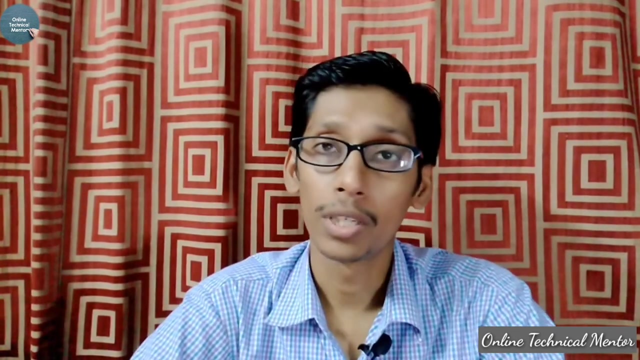 by a diagram with some specific symbol, then this diagram will be treated as flowchart. So programming is important to automate, collect, manage, calculate, analyze the processing data and information accurately, Whereas an algorithm is important in optimizing a computer program according to the available 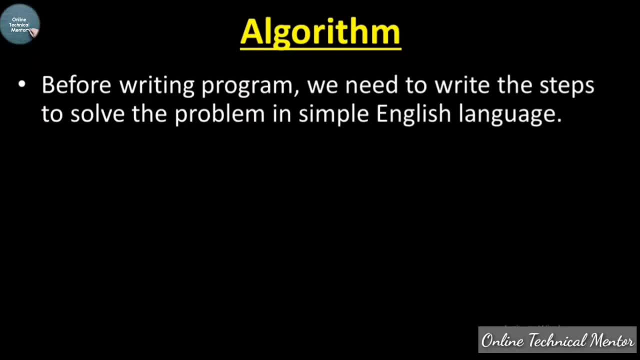 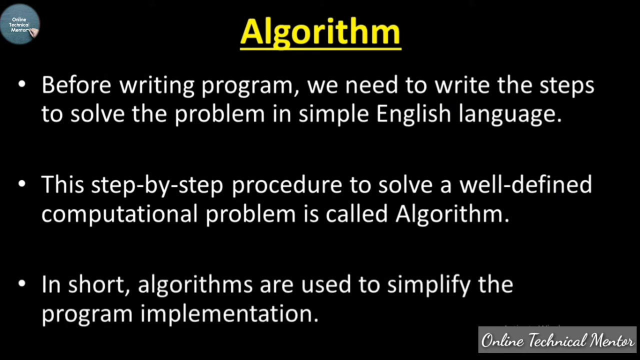 resources. Now let's summarize what is algorithm. Before writing program, we need to write the steps to solve the problem in simple English language. This step-by-step procedure to solve a well-defined computational problem is called algorithm. In short, algorithms are used to simplify program implementation. 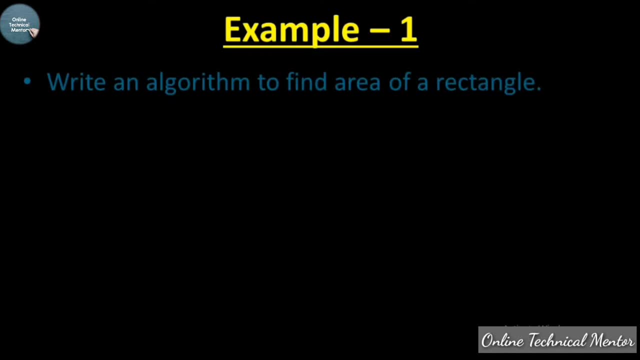 Let's see some example. first, Suppose you are given this problem, Write an algorithm to find the area of a rectangle. So what you will do: first Step 1, just write down. start Step 2, take length, breadth and store them as L and B. 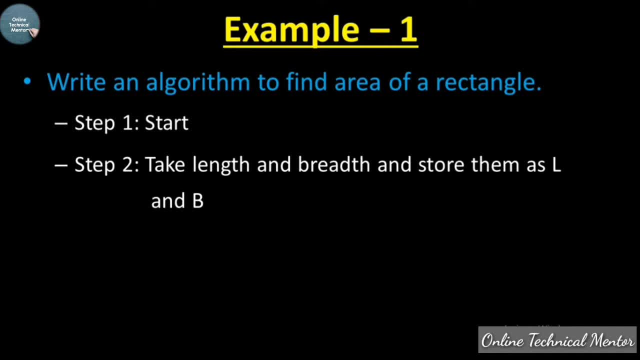 These L and B are called vectors, called variable. variable means it can store value according to users choice. so according to users choice, you can store any value within this L and B. I will explain the concept of variable in other videos. now, in the step 3, multiply L and. 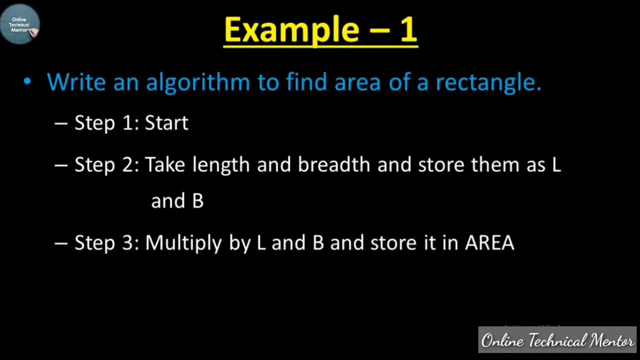 B. that's mean the value of the L and B will be multiplied and stored the result within another variable area. now print the area and at last, step 5 stop. so this is an algorithm: how to find the area of a rectangle. now you can implement this. 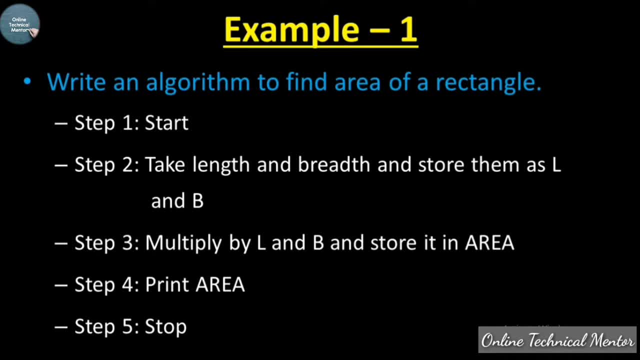 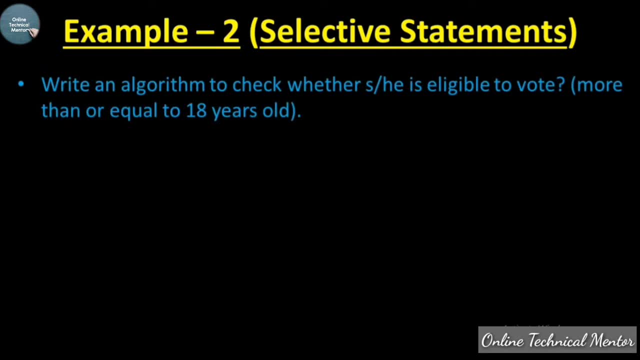 algorithm in any programming language you want. let us see another example. but there will be a selective statement. selective statement means some of the portion of an algorithm will execute an algorithm which will execute an algorithm which will execute an algorithm when others will not. similarly, when the other portion will execute the remaining, 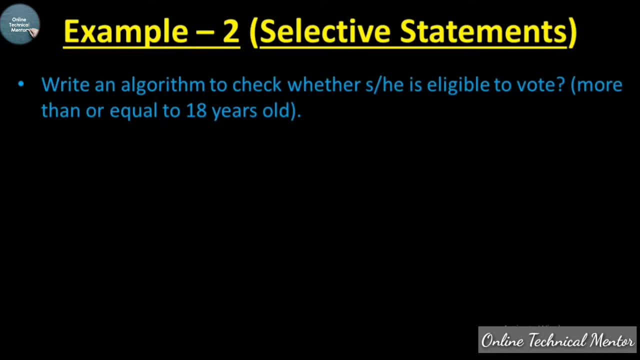 portion will not execute. write an algorithm to check whether she or he is eligible to vote. the criteria is more than or equal to 18 years old. that's mean if the person is greater than or equal to 18, he will be eligible for vote, otherwise not. so what will be the algorithm for this problem? start the. 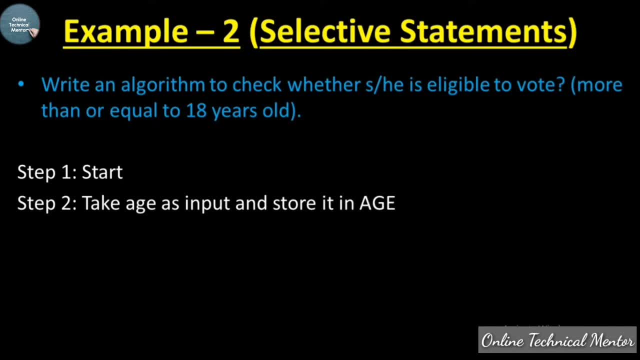 algorithm. right now. write start step 2. take age as input and store it in a variable age. now check the value of age. if age is greater than 18, then go to step 4. in step 4 it is written eligible to vote. and go to step 6. go to step 6 means after printing. 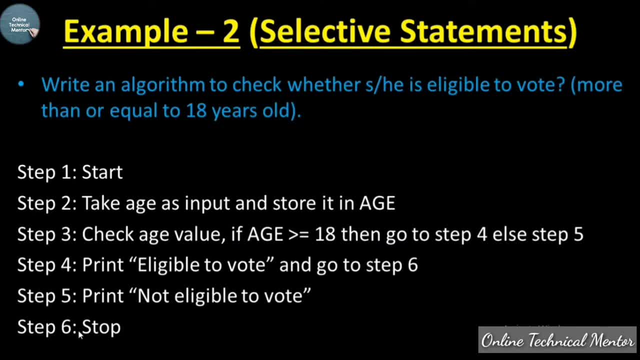 eligible to vote, the control will go to step 6. that's mean the algorithm will go to step 6. and when the algorithm will go to step 6, the control will go to step 6. that's mean the algorithm will go to step 6 and we get the result. 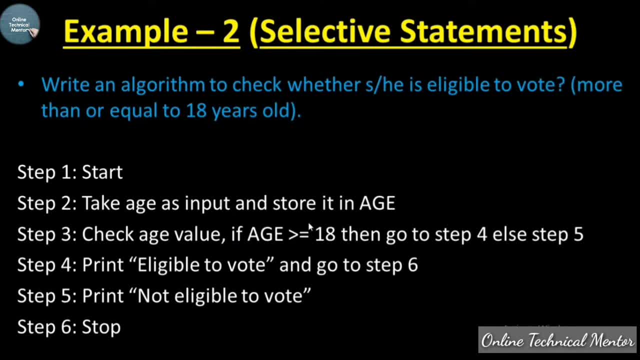 stop And if the criteria fails- that means if the age is less than 18, then it will go to the else part. That means the control will be moved to step 5.. In step 5, it is written not eligible to vote, Then it will move to the step 6.. We do not require a go-to statement at the end of step. 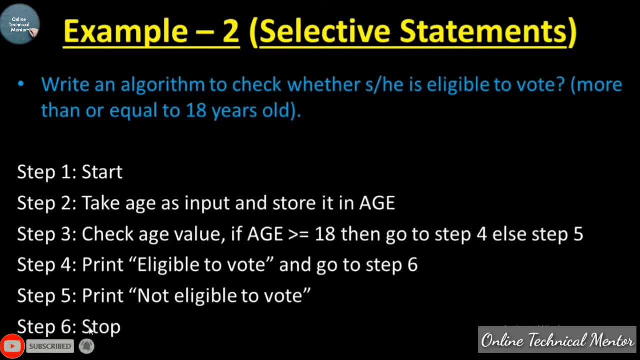 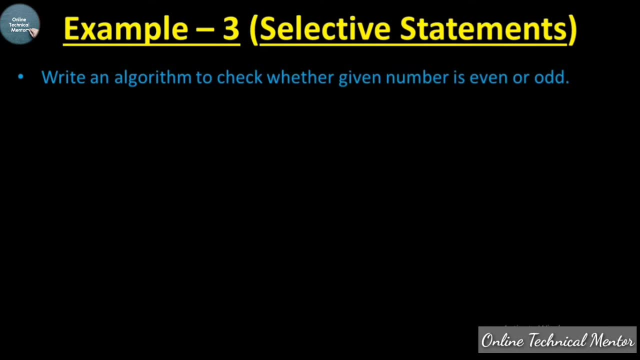 5, since the steps of algorithm execute sequentially. So after step 5, it is automatically goes to step 6.. So no need to write: go to step 6.. Let us see another example of selective statement. Write an algorithm to check whether a given number is even or odd. 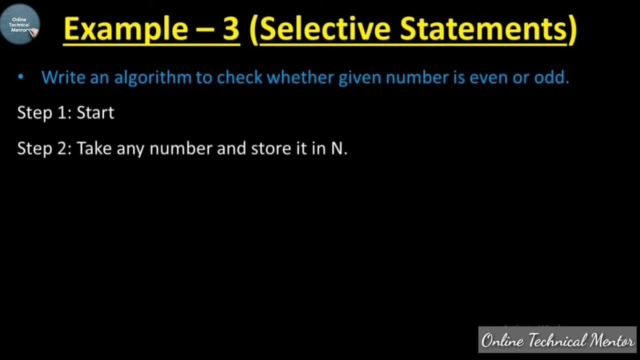 First start the algorithm. Then take any number and store it in n variable. Now calculate the result. Remember, when dividing n by 2.. So you all know that when a number is divided by 2, it will give you 0 or 1.. So the remainder will be stored within r variable, This one, this r variable. 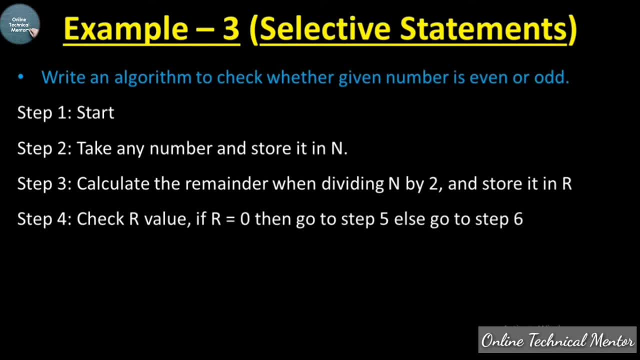 Then check the value of r. If r is equal to 0, then go to step 5.. So in step 5, it is written even number. We all know that when a number is divided by 2, it will give you 0 or 1.. So the remainder will be stored within r variable. 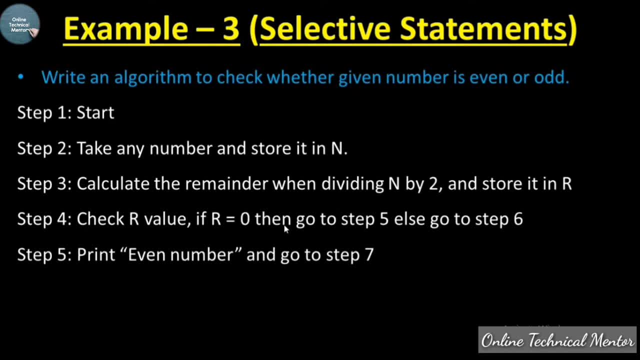 So in step 5, it is written even number, And after that it will move to the step 7, where the algorithm has been stopped. Now, if r is other than 0, that is mean when n is divided by 2- 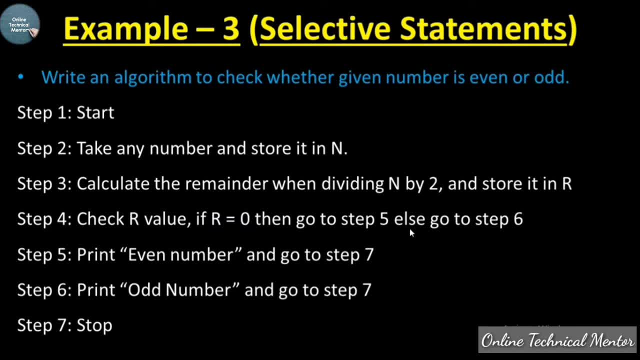 and it gives other than 0, that is mean 1. So it will move to the else part. Then the control will be moved to step 6.. So in step 6, it will give you 0 or 1. So in step 6, it will give you 0 or 1.. 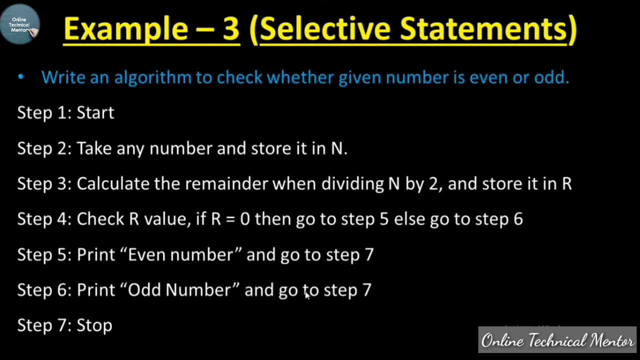 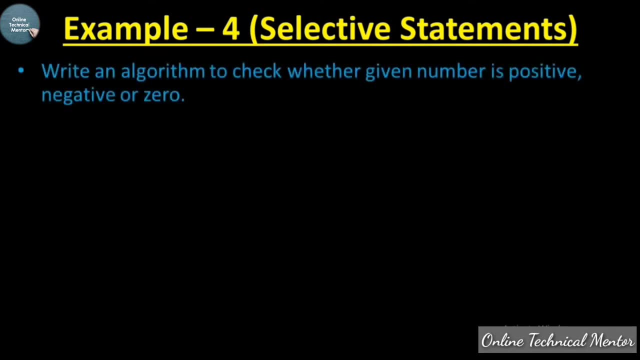 is written odd number. After that you can also write go to step 7. and if you don't write go to step 7, it will automatically move to the step 7.. Let's check another example of algorithm, and it is also a selective statement. Write an algorithm to check whether a given number is. 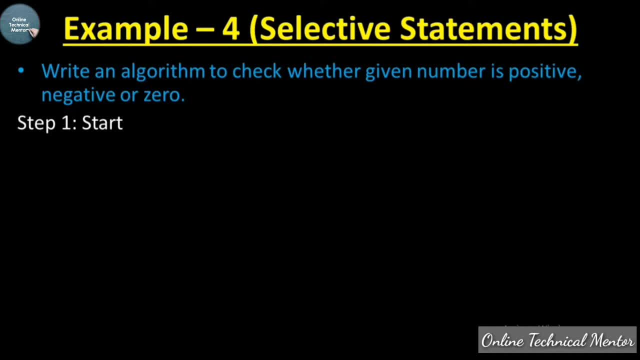 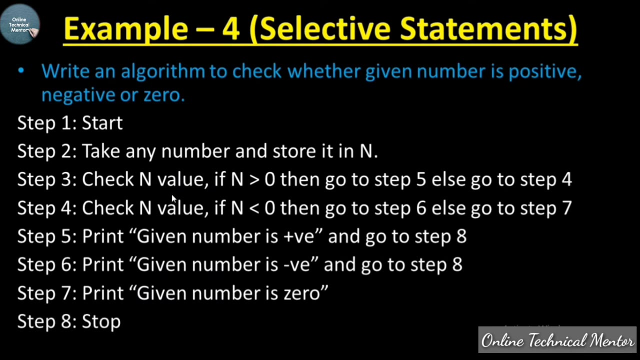 positive, negative or 0. Same as before. start the program, take any number and store it in the variable n. Now check whether the n is greater than 0 or not. Let me show you all the step. first, In step 3, check the value of n If it is greater than 0, then go to step 5.. So what is written in? 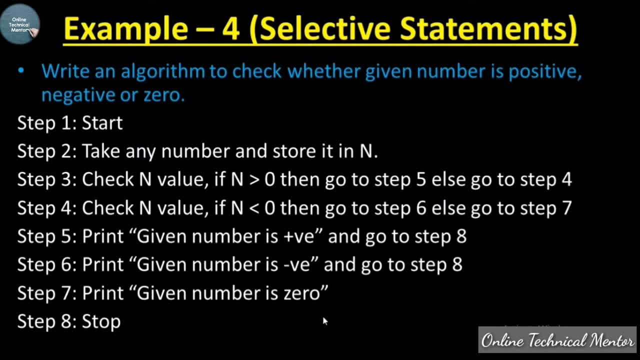 step 5? It is a positive number- and go to step 8.. Step 8 means stop the algorithm and if it is not greater than, if the n is not greater than 0, then it will move to the else part In the else. 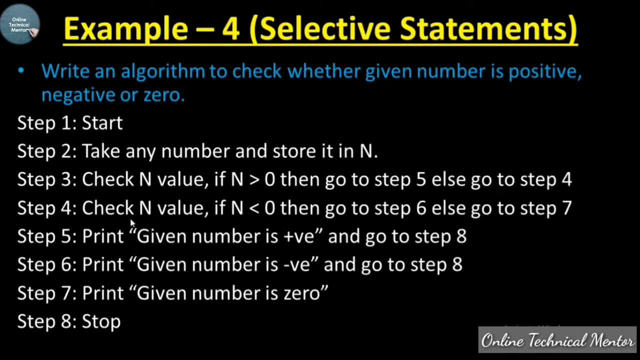 part, it will move to the positive number. So if it is greater than 0, then it will move to the else part. It is written: go to step 4.. In the step 4, you have to check the value of n again. 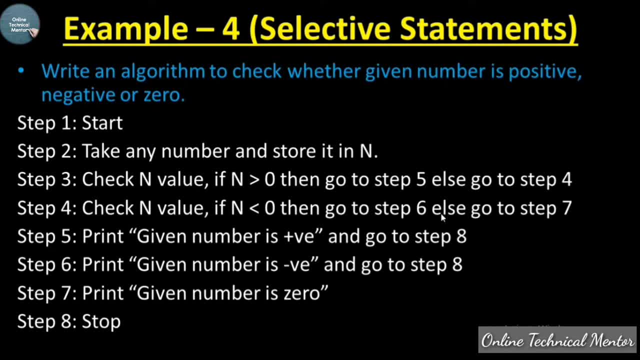 That's mean whether the n is less than 0 or not. If it is less than 0,, then go to step 6.. So in step 6, it is written: given number is negative, and then go to step 8.. So the step 8. 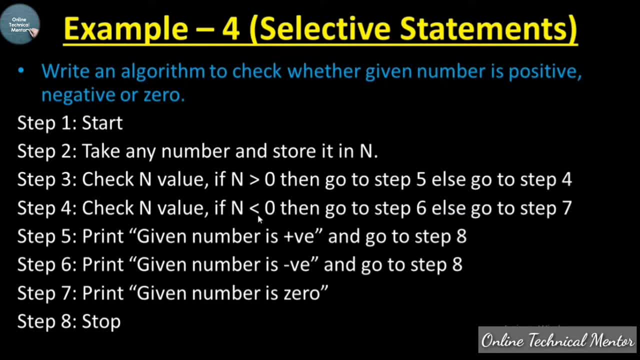 is: stop the algorithm Now in the step 4, if this condition, that is, n less than equal to 0,, if it fails, that's mean neither n greater than 0, nor n less than 0. So what will happen? It will move to the else part of step 4.. That is: 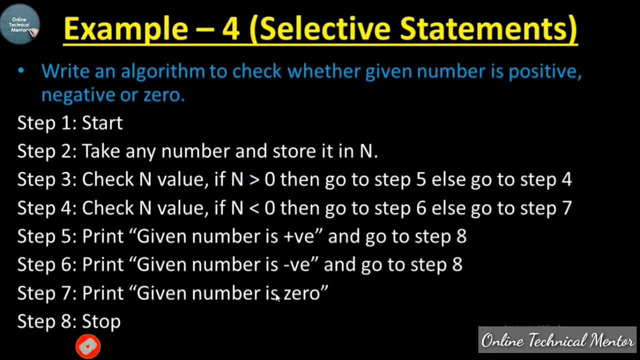 go to step 7.. So go to step 7.. It is written: given number is 0, and then it will move to the step 8.. Stop That's mean either any one of the step 5,, step 6 or step 7 is executing, That's. 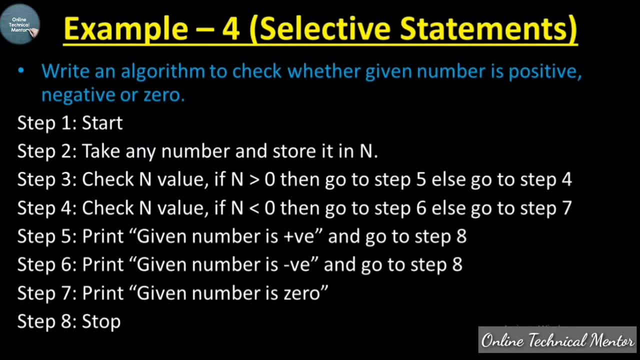 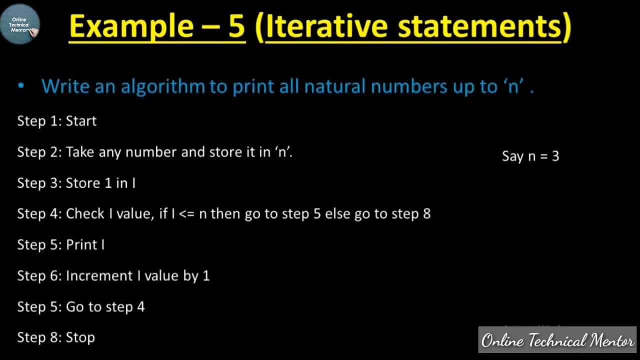 mean a portion of the algorithm is executing. That's why it is written selective statement. Selective portion of the algorithm is executing, not all. Now here is a different example of an algorithm. It is an iterative statement. Iterative statement means when some portion of an algorithm will execute again and again. 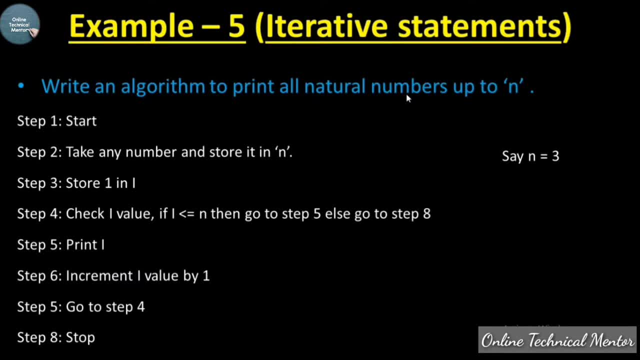 Look, write an algorithm to print all numbers up to n. Suppose you have given the value of n as 3.. That's mean it will print 1,, 2, 3.. Let's check. Start the algorithm, Take any number and store it. 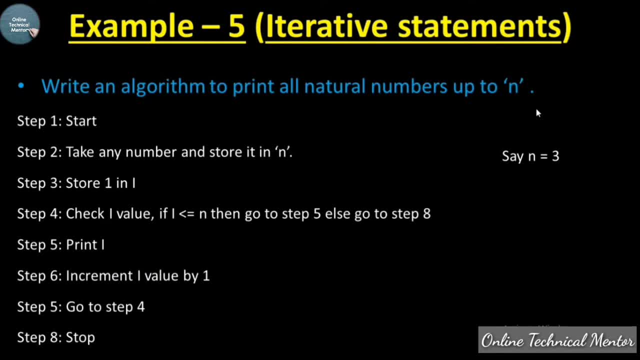 in n. That's mean you have to take input from user. Say, I have taken n equal to 3 in my example. The next step initialize i with 1.. That's mean I have written. store 1 in i. That's mean i will. 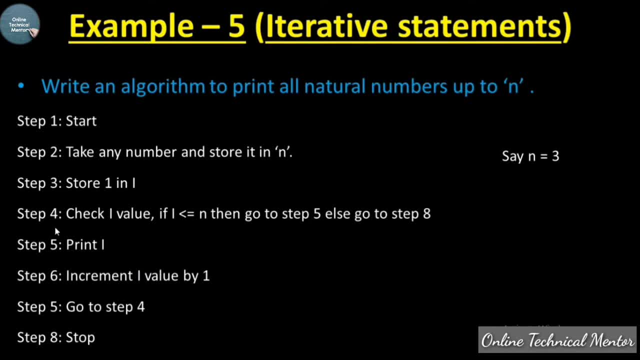 be initialized with 1.. In the step 4, check i value. That's mean the initial value is 1.. So 1 less than equal to n. Is the condition correct? 1 less than equal to 3.. Since n is 3 in my example and i is initialized with 1 initially. 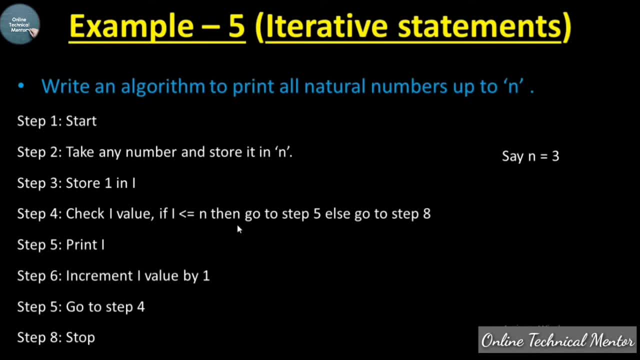 So 1 less than equal to 3.. If it is satisfied, then go to step 5.. Yes, for the first case it will satisfy, Go to step 5.. In the step 5, it is written print i. That's mean 1 will be printed. 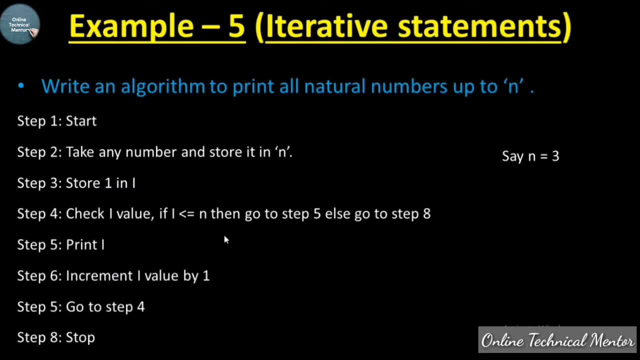 in the output screen. After that I will be incremented by 1.. That's mean i was initially 1 and now it will become 2.. In step 5, go to step 4.. Again, the control will be moved back to the step 4.. Now the present value of i is 2.. 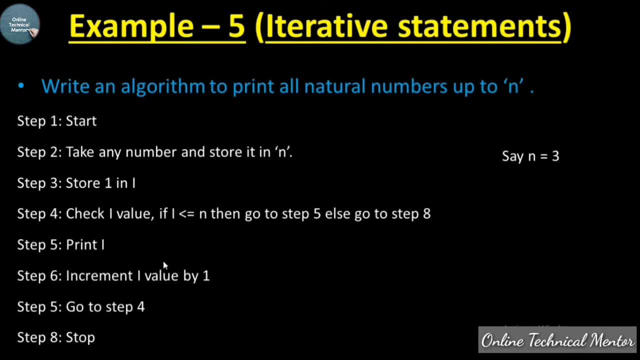 Now 2 is less than equal to 3.. Yes, Then again go to step 5.. Next, print i. It will again print 2. so after 1, it will print 2. then again, increment the value of i by 1. that's mean now: 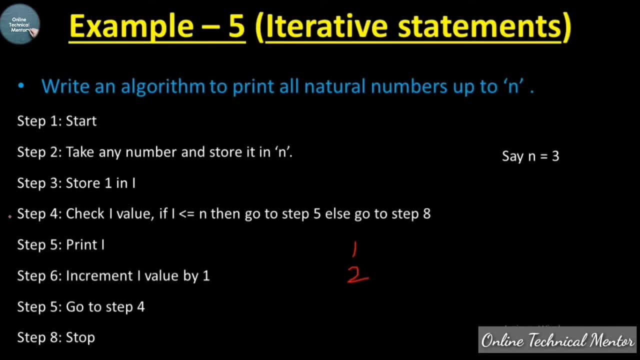 i will become 3 again. go to step 4. control will move to step 4. the present value of i is 3, now 3, less than equal to 3. it is not less than, but equal to 3. then again it will go to step 5 condition. 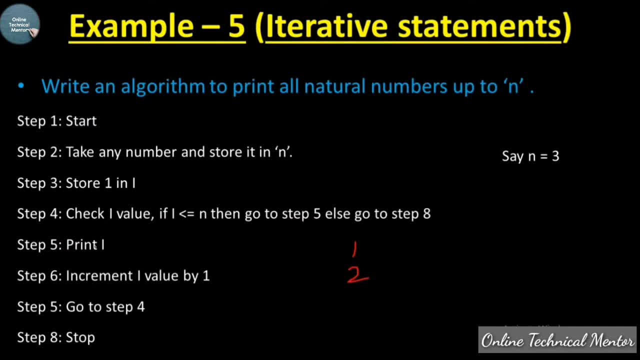 is true, so it will move to step 5. so in step 5 there is print i, so the new value of i will be printed. that is 3. next step 6: increment i value by 1. so i will be again incremented by 1, that's. 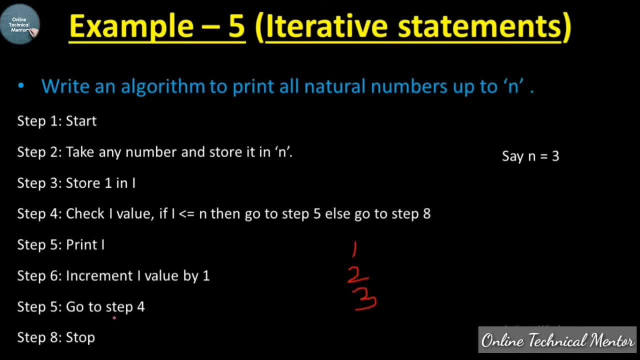 mean i will become 4 this time. now go to step 4. the control will be moved back to step 4. now the present value of i is 4, so it will move to step 5. so in step 5 there is print i, so the new value of i will be printed. 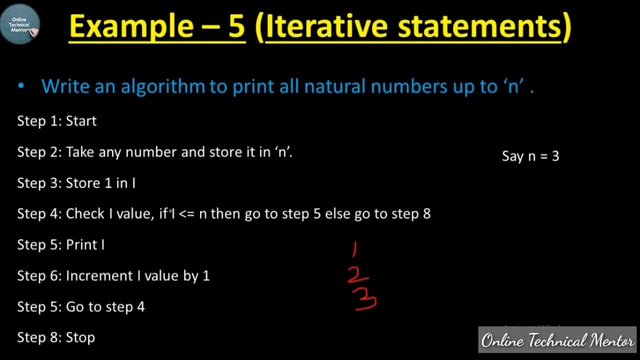 and since n is 3, it is a constant. now 4 less than equal to 3. no, 4 is neither less than nor equal to 3, so it will move to the step 8. that's mean step 8, stop the algorithm. so in the meantime, 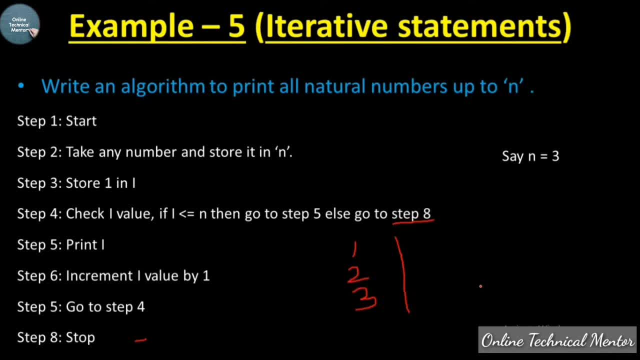 it will print all the natural number from 1 to 3. so these are some basic example of algorithm. by using this algorithm you can now write program in any programming language, whatever may be the size of your program, whatever may be the complexity. i will suggest you write the algorithm first, then write your program. i think it will be better for 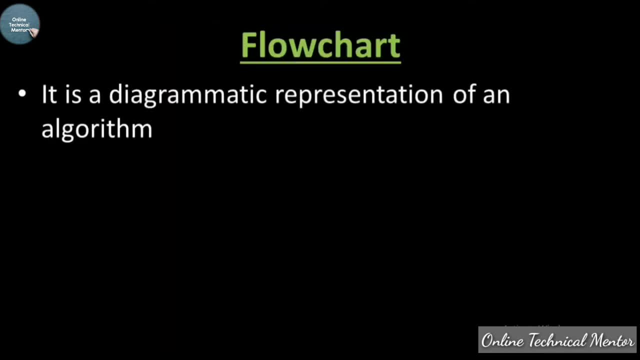 you now come to flowchart. it is a diagrammatic representation of an algorithm. a flowchart is a type of diagram that represent a workflow or process, a step-by-step approach to solve a task by using some algorithm, and then you can write the algorithm first, then you can write the algorithm. 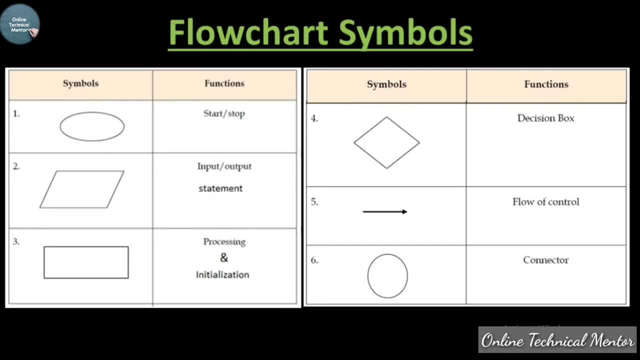 symbols. So what are the symbols? Let's check. So these are some symbols that we are going to use in a flowchart. The first one is the oval shape. It represents start or stop of a flowchart, Then a parallelogram. It will be used in case of input-output statement. 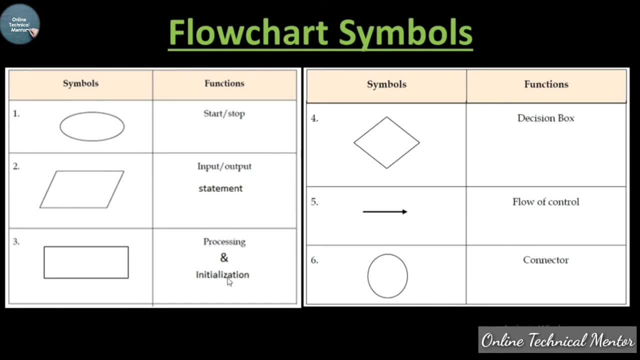 A rectangle box. It will be used in case of processing and also in case of initialization. also. Number four is a rhombus. This will be used in case of decision, Suppose A greater than B or A not equal to B. This kind of decision will be written within this rhombus. Next, number five. 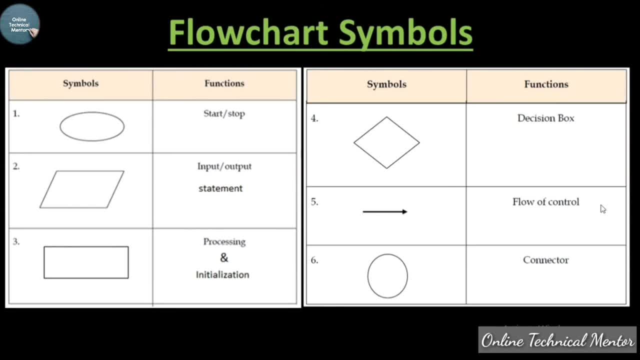 this arrow will be used for flow of control, So it can be up arrow, down arrow, left arrow, right arrow, And this is a connector. When you are drawing a flowchart, it may happen that you can't accommodate the whole flowchart within a circle. So you can't accommodate the whole flowchart. 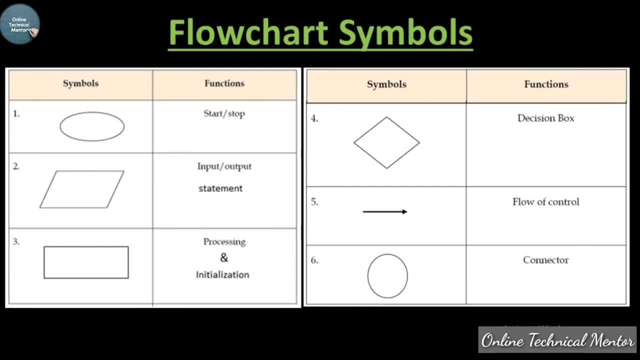 within a circle, So you can't accommodate the whole flowchart within a circle, So you can't have a single page, So you have to move to the other page also or in the next page. So by using this connector you can connect the ending and starting point of two different portion of that. 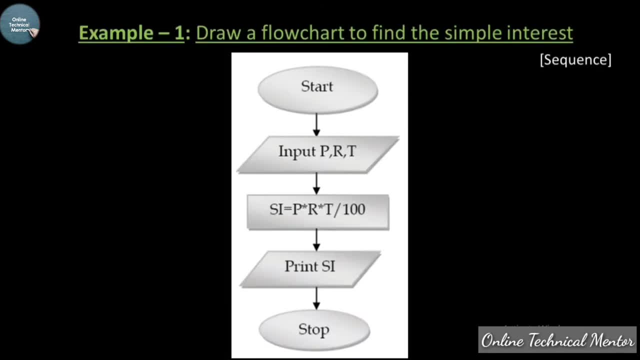 flowchart. Now let's see some example of flowchart. Suppose you are told to draw a flowchart to find simple interest. So what you will do? Start the flowchart. Next you have to take input for principle, rate and time. 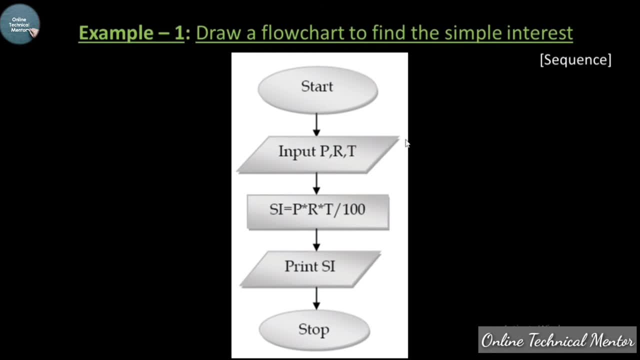 So, since it is an input statement, enclose it within a parallelogram. Then find the simple interest by using the formula principle into rate, into time divided by 100, and store the result into the SI variable. So when there is an assignment operator, the right-hand side of the assignment. 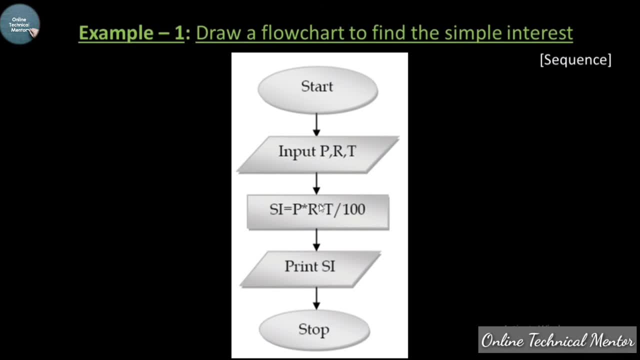 operator will execute first and the value will be stored at the left-hand side. So now SI will store the simple interest calculated from the given PRT. After that, move to the flowlines. Flowlines is showing downward. Now print the variable SI. After that stop the flowchart. So this is a 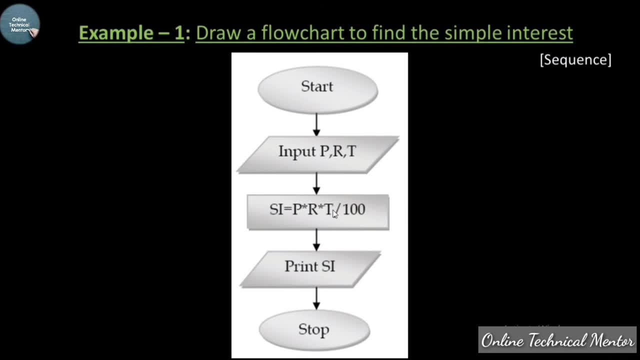 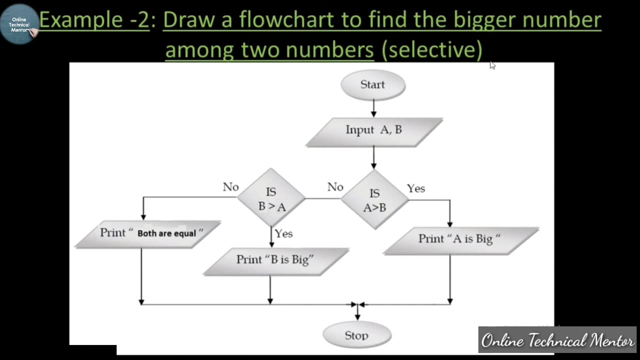 sequence- flowchart. Sequence means one instruction is after another, So it is moving in a downward direction. Let's look at another example. It is equivalent to a selective statement. It is a selective flowchart. Draw a flowchart to find the bigger number among two numbers. Start the program. 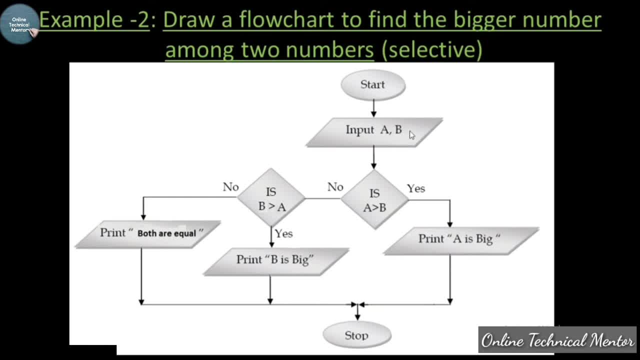 Take two values from user and store it within A and B. So I have written input A, B And since it is an input statement, it is enclosed within a parallelogram. Now move to the downward. This is a flowline. 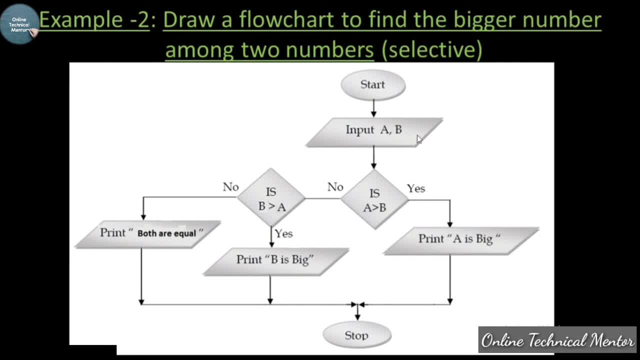 So here is a decision box. So you have to take decision whether A greater than B or not. So you have to write like this: is A greater than B? You can give also a question mark over here. So a decision box has one input line and two output line. So this is an input line. It has a two output. 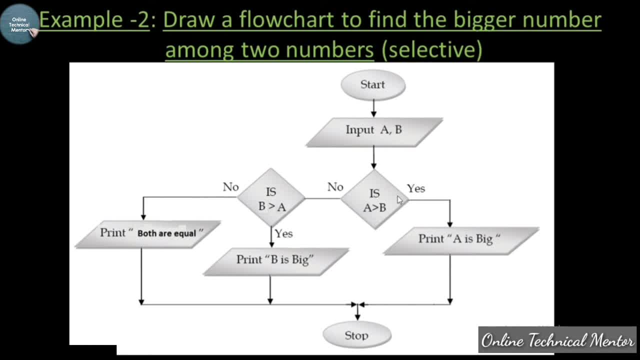 line One is yes and another is no. You can also write true or false. If it is true, that means if the answer is true, we move to the right hand side. Here it is written: print A is B. Since this is a print, 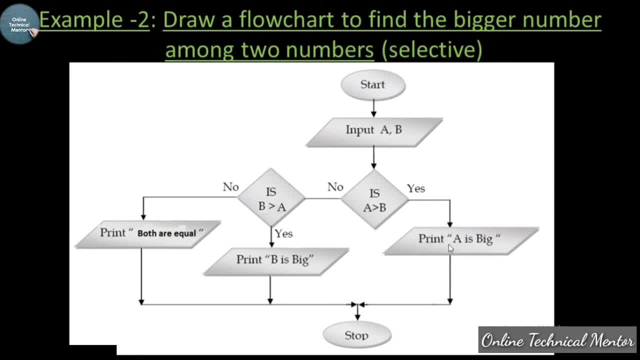 statement. input statement. it is always enclosed within a parallelogram. After printing this line it will move to stop. Suppose A greater than B. if the condition is false, then it will move to the no part. So in the no part. 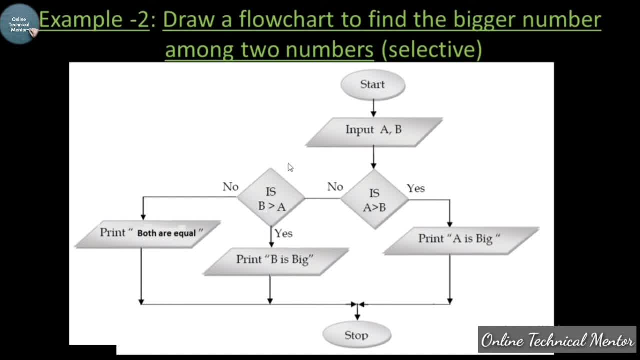 it is, again encounter a different dossier box, But there is another checking whether B is greater than A or not. so again, there will be two output from this decision box. one is yes and another is no. if the condition is true, then it will move to the yes part and it will print. 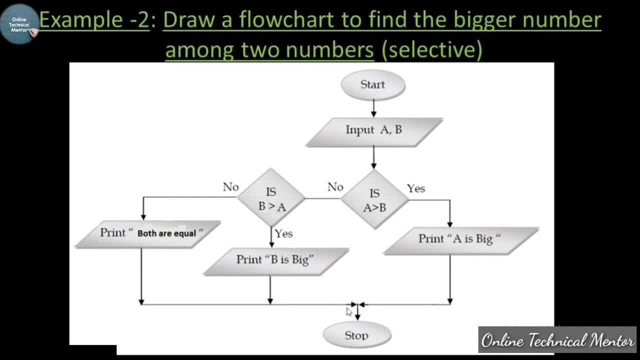 b is big. after printing b is big, it will move to stop. and if this condition is false, that's mean a greater than b false. so it's moved to this decision box again: b greater than a. this condition is false. so again it will move to the no part. it will print: both are equal and since it is a, 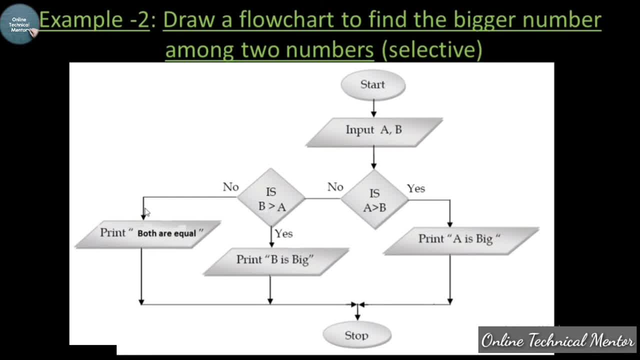 printing statement. it is enclosed within a parallelogram. after printing this, it will again move to stop. i think you have realized that not all the portion of this flowcharts are executing. either this one is executing. either this one is executing or this one, so that is why i have written selective. 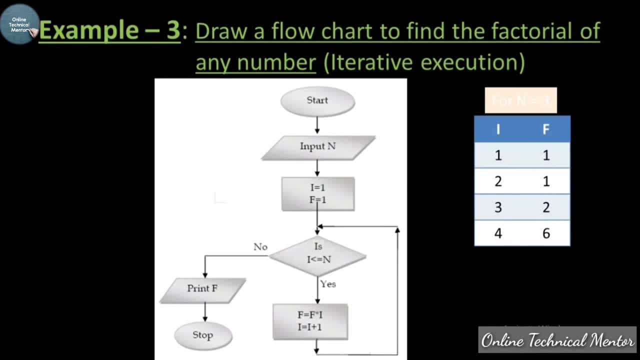 let's check another example. it is called iterative execution. why iterative execution? because a portion of the flowchart will be repeated again and again. draw a flowchart to find the factorial of any number. i think you all know about the factorial. the factorial of three is one into two into three. the factorial. 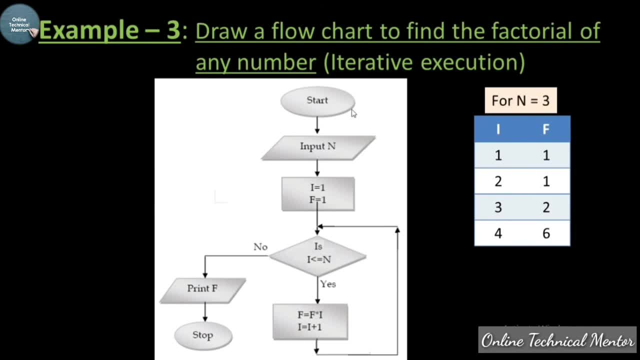 of four is one into two, into three, into four. start the flowchart. accept any values for factorial. so within parallelogram, right input n, suppose i have taken n equal to 3 for an example. now initialize i with 1 and f equal to 1. i is a counter variable and the f variable will store. 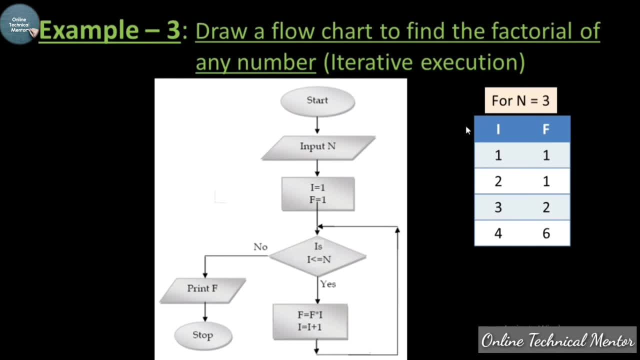 the factorial of the given number n. look at the right hand side. i have drawn a chart where the value of i and f has been shown. so initially, both the value of i and f is 1.. so i've written one one in place, that's 1 in. 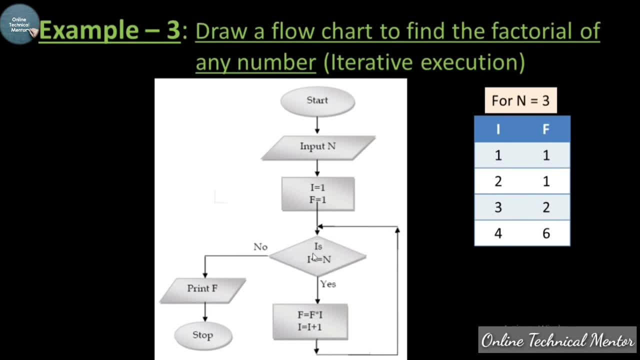 of i and f. So in the decision box check whether the value of i is less than equal to n. Now the initial value of i is 1 and the n is 3.. 1 is less than equal to 3.. Yes, 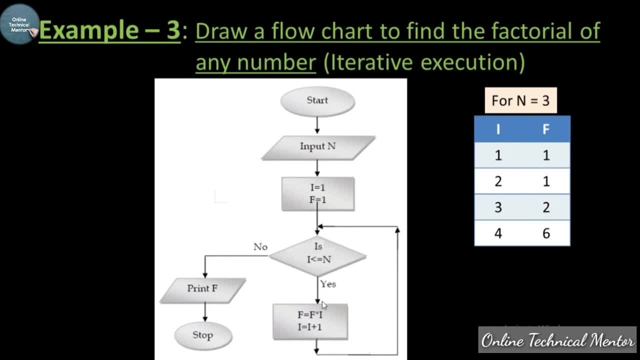 the condition is true, Then it will move to the yes part, And in the yes part there is a processing box where it is written f equal to f into i. That means f will be multiplied with i and the value will be stored within f. Look at the table. 1 will be multiplied with 1. 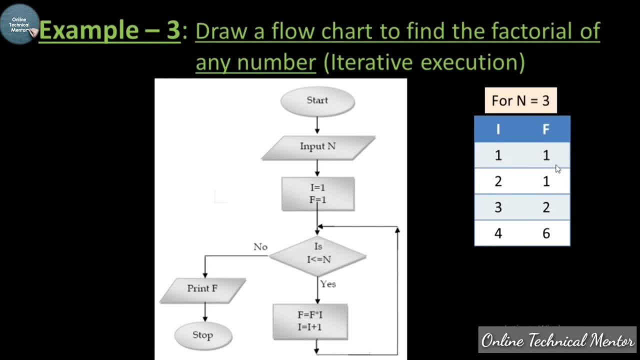 and that will be stored within f. In the next line i will be incremented by 1.. Now i will become 2.. After this it will automatically move to the beginning of this decision box. So again, it will enter into this decision box. 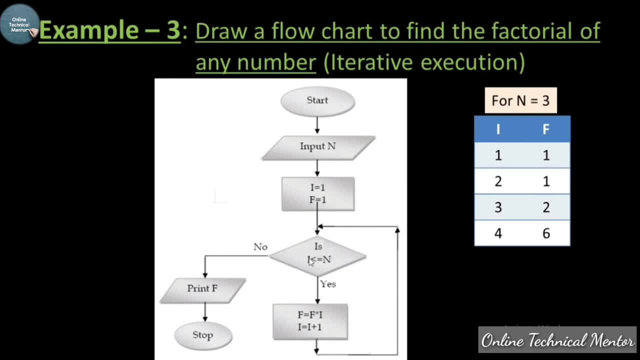 This time the value of i is less than equal to 3 and i will be stored within f. i is 2.. Now again it will check with n. That's mean 2 is less than equal to 3, or not? Yes? 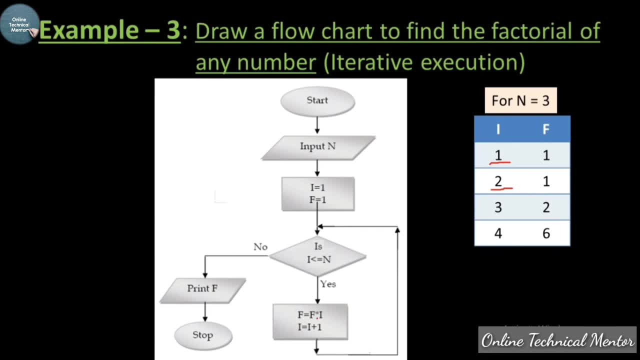 it is correct. So just move to the processing box. Again, multiply f with i. That's mean the present value of f is 1 and this will be multiplied with i, that is 2, and it will give you the new value of f2.. Again, the control will move upward. Again it will enter into. 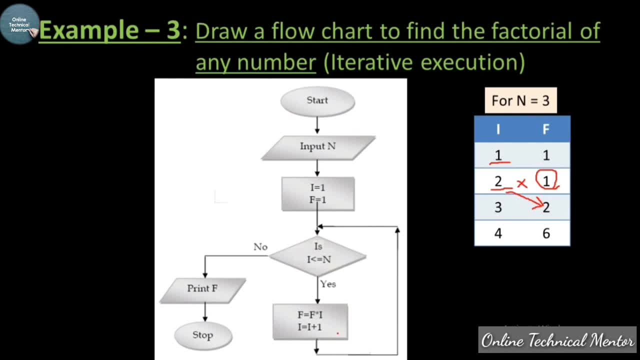 the decision box, Then i will be incremented by 1.. So now i will become 3.. Then the control will be again. move upward and enter into the decision box. This time the value of i is 3.. So it will check with n. That is, 3 is less than equal to 3.. Yes, it is equal to. 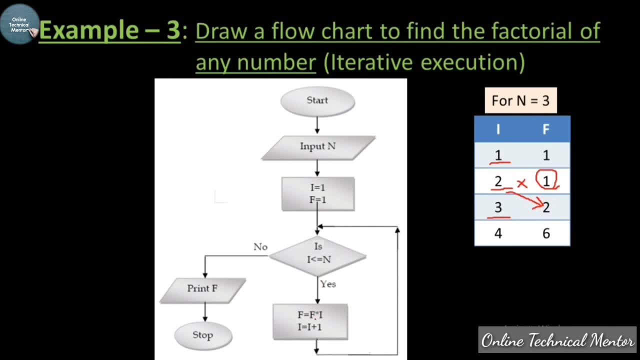 3.. Again it will move to the yes part. Now the f will be multiplied with i. The present value of f is 2.. So this 2 will be multiplied with the present value of i, that is 3, and it will. 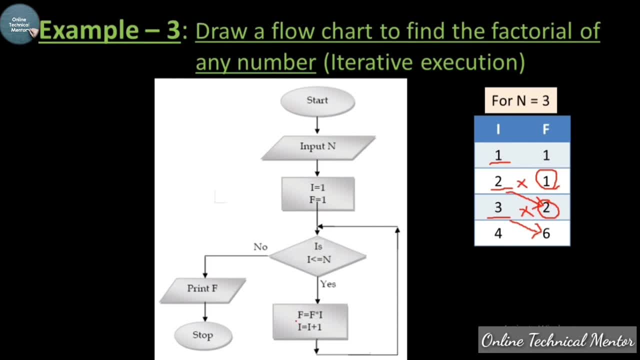 give you a 6.. So this 6 will be stored within f. Next, i equal to i plus 1.. Again, i will be incremented by 1 and it will become 4.. Again, the control will move upward and again it will enter. 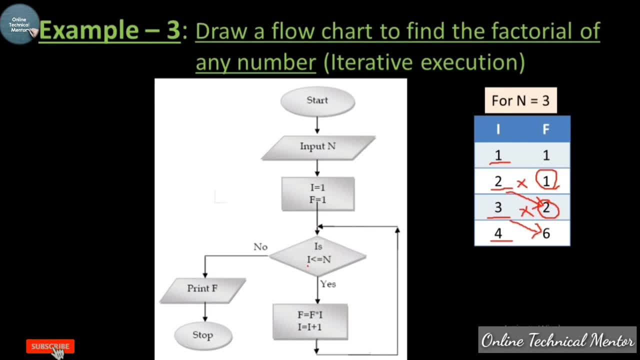 into the decision box. This time the value of i is 4.. Now when it will check with n 4 less than equal to 3, no, This time the condition will become false And the control will move to the no part. 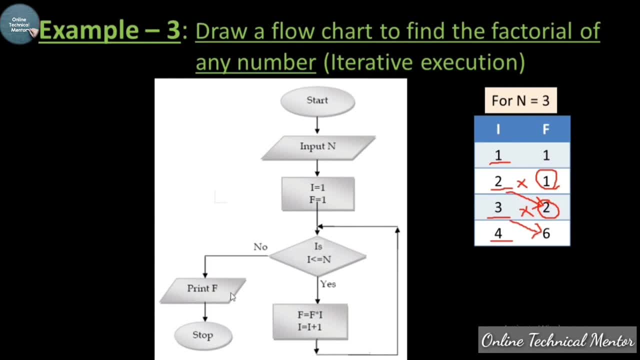 So in the no direction there is an output statement printf. So this time the value of f is 6,, which is the factorial of 3.. so it will print the factorial of three and then the flowchart will stop. so before designing a program, you can either write an algorithm or draw a flowchart. it's up to you. 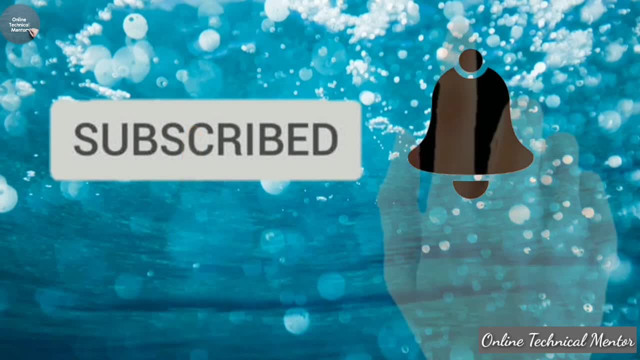 subscribe to my channel online technical mentor and press the bell icon for latest update. thank you.